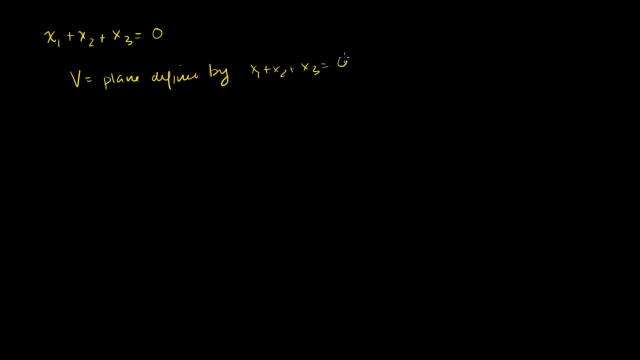 x1 plus x2 plus x3 is equal to 0.. All of the vectors in the subspace: if you take their entries and you add them up, you're going to get 0.. So first we need just any basis for v. so let's see if we. 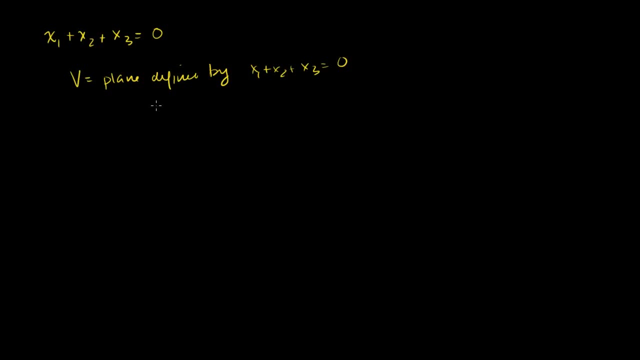 could come up with that. So if we subtract x2 and x3 from both sides of this equation, we know that x1 is going to be equal to 0.. x2 is equal to minus x2 minus x3.. Or we could say that our subspace v is equal to the set. 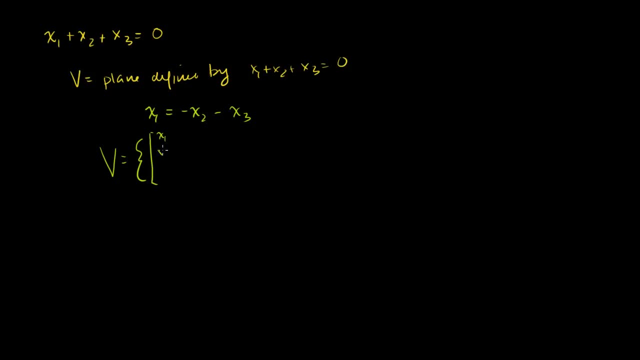 of all of the vectors in R3,, x1,, x2, and x3, that satisfy the equation. let's say minus. let me write it this way: Let's say that x2 is equal to c1 and x3 is equal to c2.. 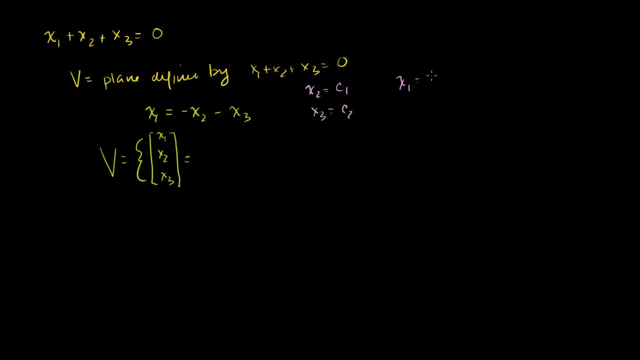 Then this equation would be: x1 is equal to minus c1 minus c2.. So if we write it that way, then the subspace v is the set of all of the vectors in R3, such that c1 times some vector. Let me write it this way: 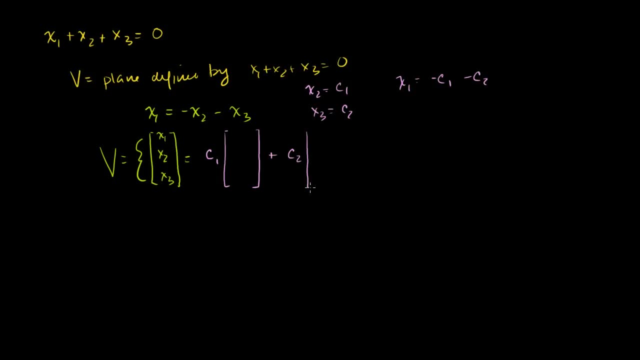 x1 is- let me write it this way- plus c2 times some other vector where c1 and c2 are any real numbers. so c1 and c2 are real numbers. So this is x1 times c2, so let's see: x1 times c2 and c3 are: 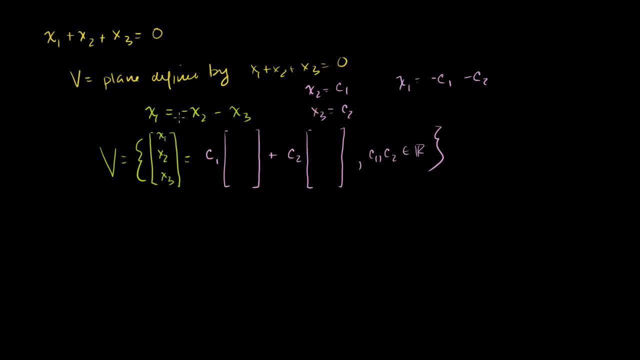 are a member of the reals. And so what is x1?? x1 is equal to minus c1, minus c2.. So x1 is equal to minus 1 c1, minus 1 c2.. x2 is just equal to c1.. 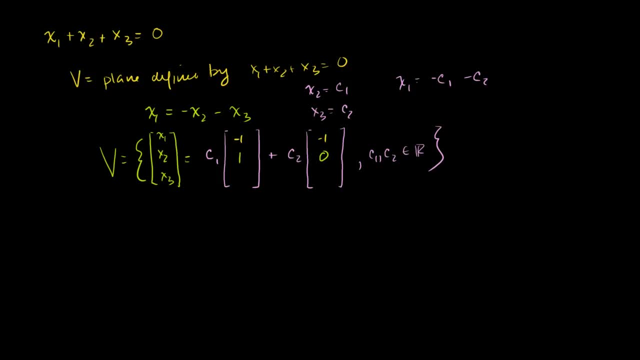 So x2 is equal to 1 times c1 plus 0 times c2.. And then x3 is equal to c2, or 0 times c1 plus 1 times c2.. So v is essentially the span of these two vectors, all of. 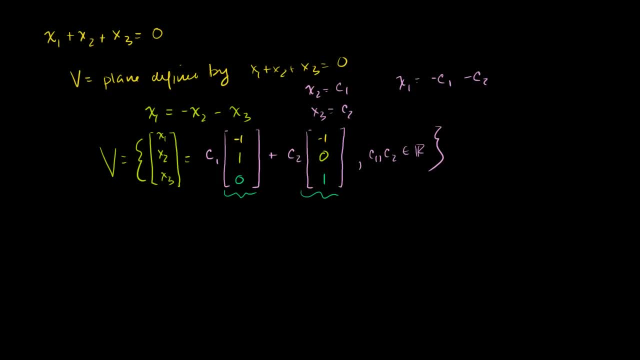 the linear combinations of these two vectors That would represent that plane. So let me write it like this: v is equal to the span of the vectors minus 1, 1, 0, and the vector minus 1, 0, 1.. 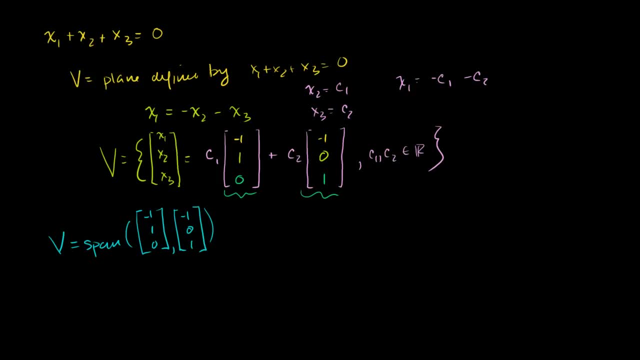 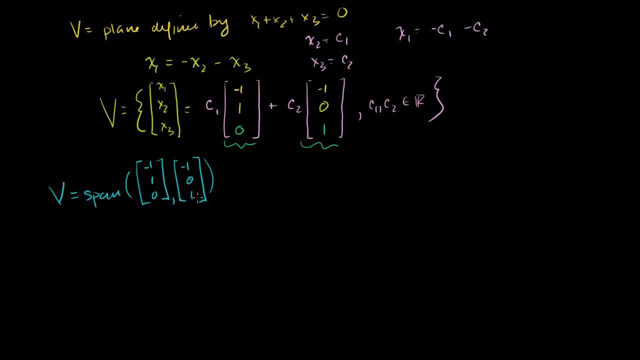 And you can see that these are linearly independent. Obviously, there's no linear combination of this guy that can give you a 1 over here. There's no linear combination of this guy that'll give you a 1 right there. So this is what v is. 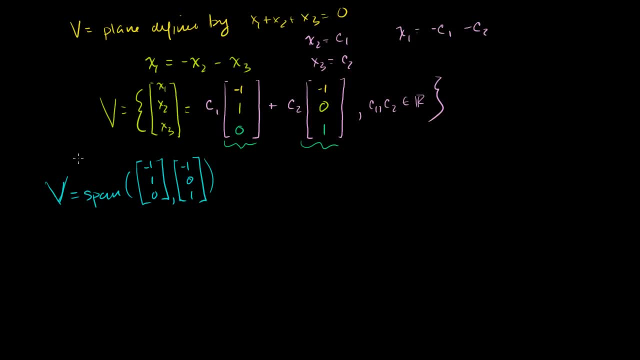 But what we want, the whole reason why I'm making this video- is to find an orthonormal basis for v. This is just a basis. These guys right here are just a basis for v. Let's find an orthonormal basis. 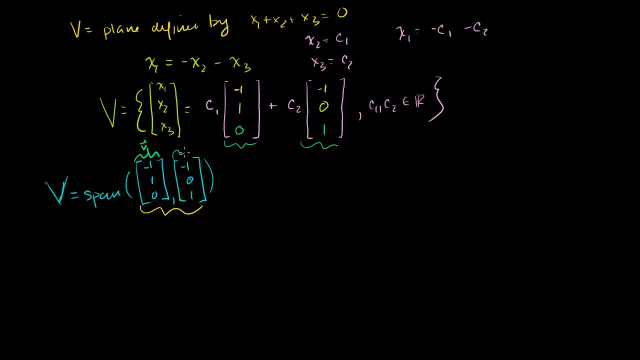 Let's call this vector up here, let's call that v1, and let's call this vector right here v2.. So if we wanted to find an orthonormal basis for the span of v1.. Let me write that down. Let me define sub-subspace: v1 is equal to the span of just my. 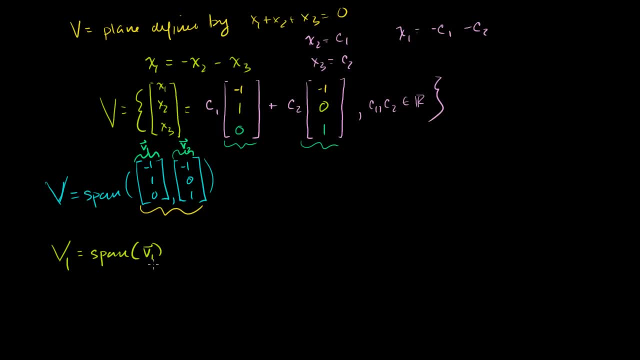 vector v1.. Well, we saw in the last video, if we just divide v1 by its length, then we'll have the span of that vector is going to be a unit vector and it's going to be the same thing as the subspace v1, as this line in R3.. 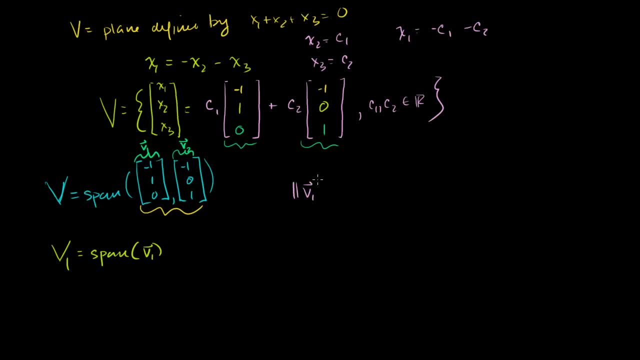 So let's do that. What is the length of v1?? The length of v1 is equal to the square root, The square root of v1.. Let me write this down: The square root of minus 1 squared, which is 1, plus 1. 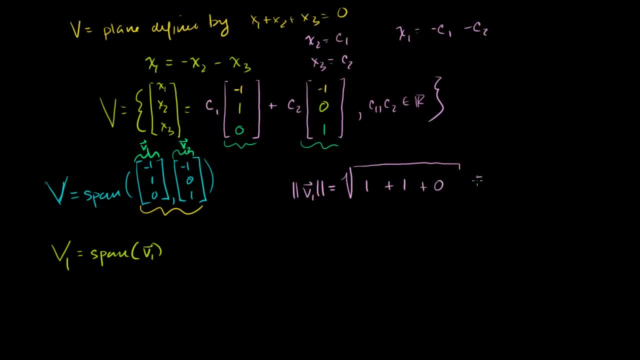 squared, which is 1, plus 0 squared, which is 0.. So it's equal to the square root of 2.. So let's define some vector. u1 is equal to 1 divided by the length of v1,. so 1 over the square root of 2, times v1,. 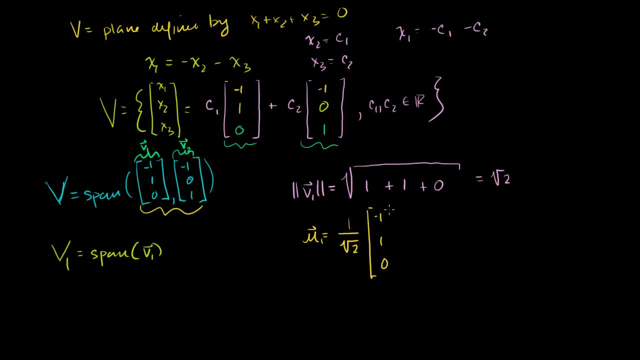 times minus 1, 1, 0. Then the span of v1 is just the same thing as the span of u1. And so this would be an orthonormal basis. Just this vector right here would be an orthonormal basis. 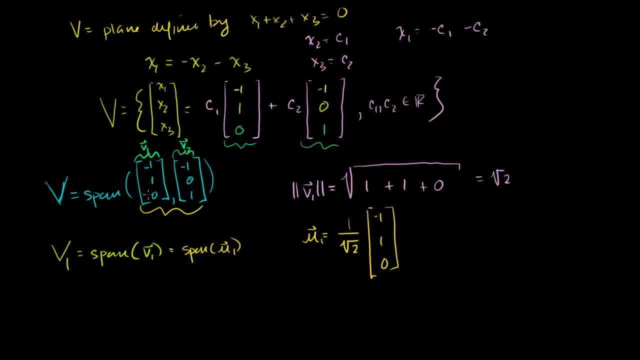 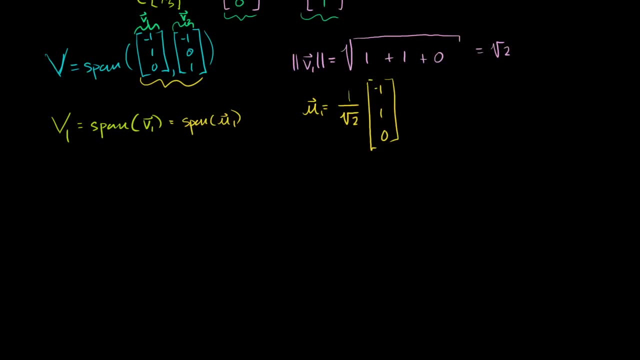 for just the span of v1.. But we don't want just the span of v1. We want the span of v1 and v2.. So let me draw it. So right now we have a basis. If I just do u1, I'm not going to actually draw what this. 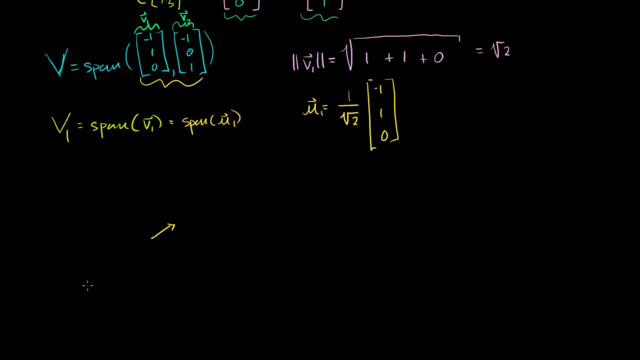 looks like. maybe it looks something like this And its span is this entire line in R3.. So its span is this entire line. The span of just one vector in Rn is just going to be all the scalar multiples of it, or a line in Rn. 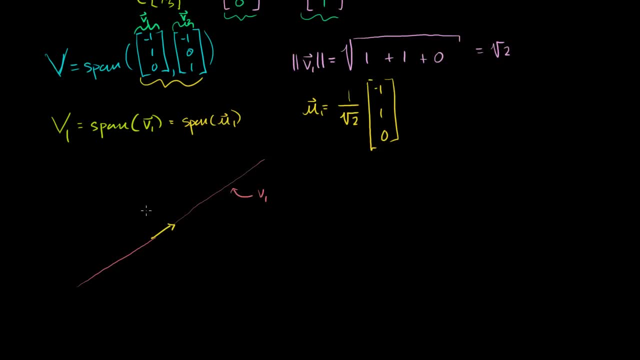 So this right here is the subspace v1.. Now we have a v2 here which is linearly independent from this guy. which means it's linearly independent from this guy because he's just a scaled version of this guy. So v2 is going to maybe look like that. 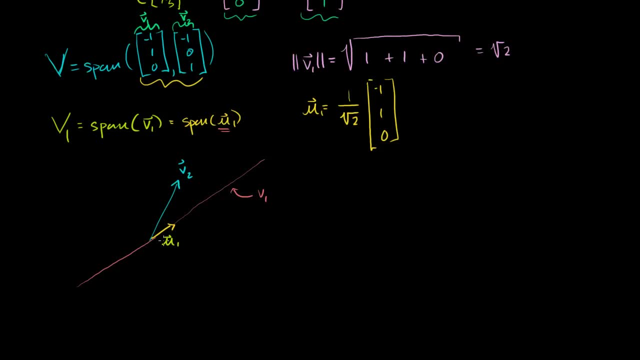 That is v2, right there. This, of course, was our u1.. What we want to do is we want to define a subspace v. I'll call it v2 for now, but it's going to be. v2 is equal to. 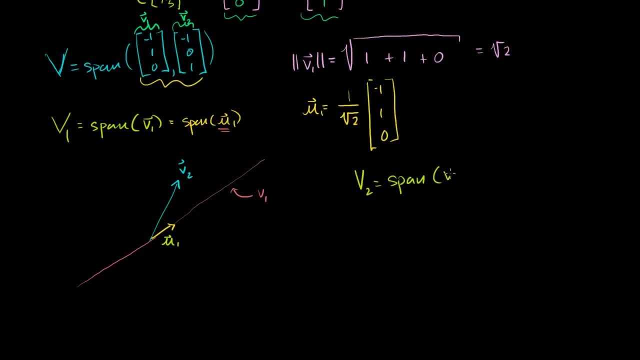 the span of v1 and v2, which is the same thing as the span. Anything that's spanned by v1 is also spanned by u1, as the span of u1 and v2.. So we want to see everything that can be generated by linear. 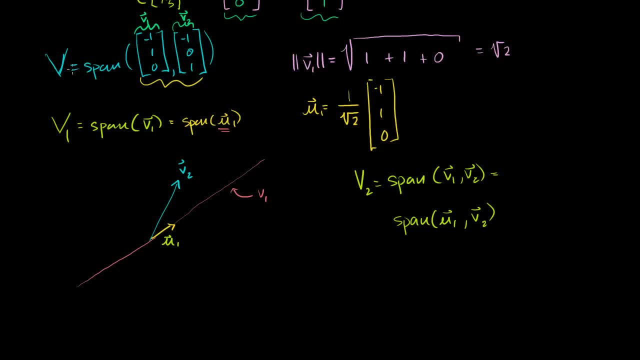 combinations of u1 and v2.. And obviously this thing right here is our plane, that we're talking about. the span of these two guys. That is the whole subspace that we're talking about in this problem. So that is equal to v. 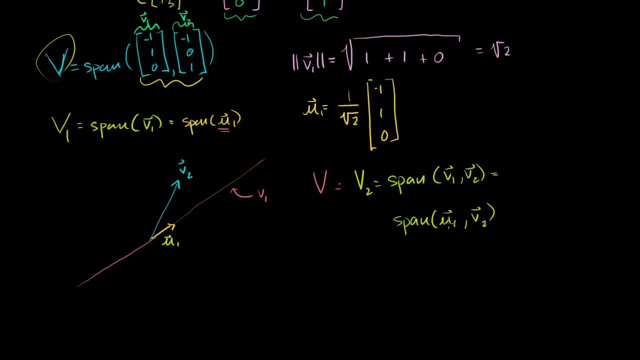 So once we find this, if we find an orthonormal version for this span, we're done. So how can we do that? Well, if I can find a vector that's orthogonal to all of the linear combinations of this, that if I add up some 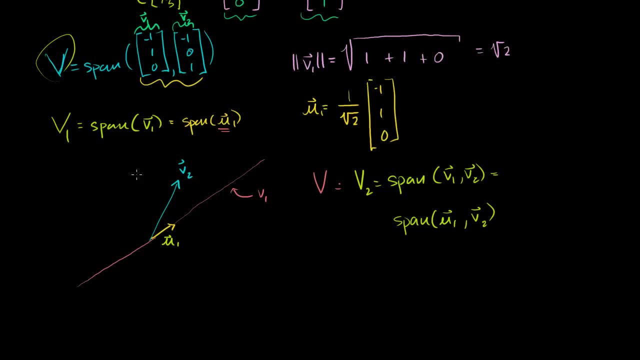 linear combination of this to that vector. I can get v2,. I can replace v2 with that vector, So we could call that vector right there y2.. If I can determine a y2, this y2 is clearly orthogonal to everything over here. 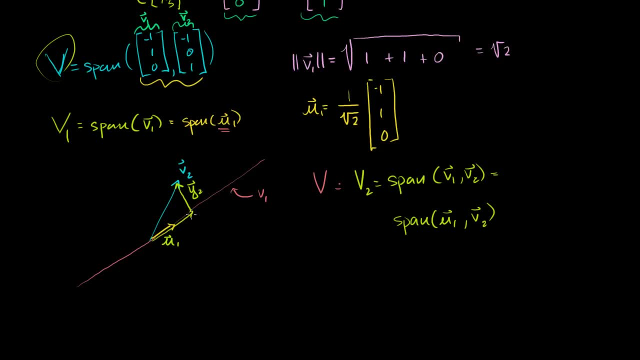 And I can take some vector in v1 in this line and add it to y2, and I can get to v2.. So the combinations of these guys are just as good as v2.. So this is going to be equal to the span of u1 and y2.. 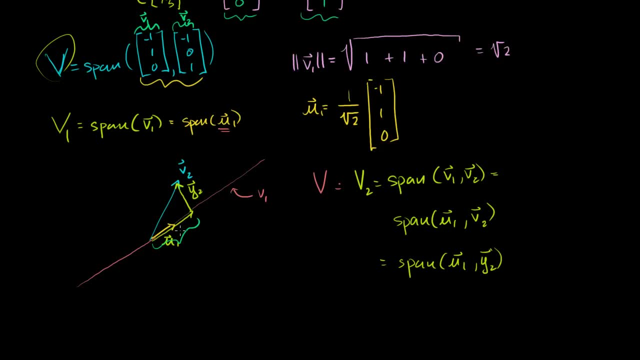 Now, what is y2 equal to? Well, we saw in the last video, this is just the projection of v2, this vector right here is the projection of v2 onto the subspace v1.. And how do we figure that out? Well, you can do that by taking some vector in v1 and adding. 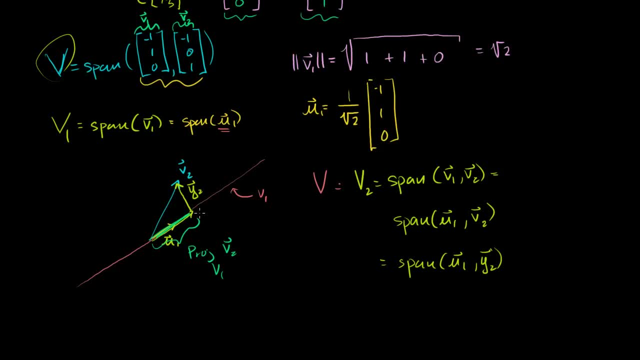 it to y2.. Figure out what that is. and then what would y2 be? y2 would be v2 minus that, So y2 is equal to v2 minus the projection of v2 onto v1.. Or if we were to actually write it out, what is that? 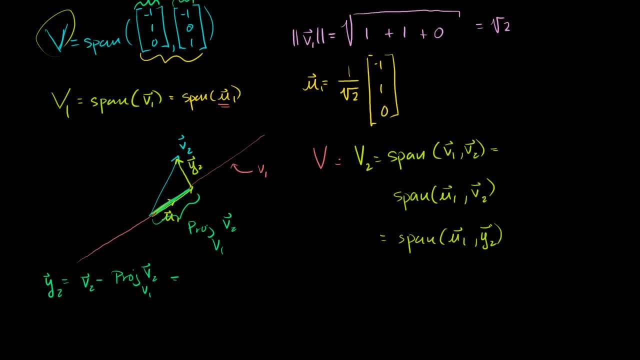 going to be equal to. So it's going to be equal to v2. is this vector right here? So it's minus 1, 0, 1.. That is v2.. v2 minus the projection of v2 onto v1.. 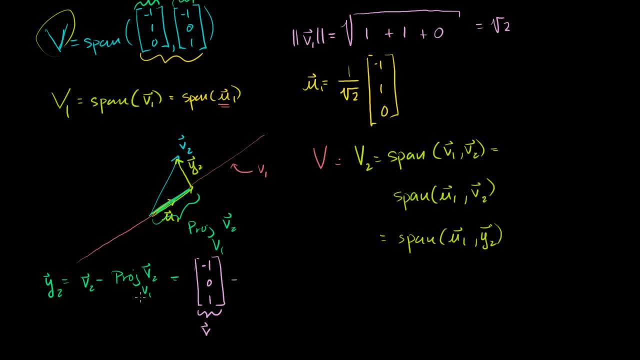 Well, the projection of the vector v2 onto the subspace. v1 is just v2, minus 1, 0, 1, dotted with the orthonormal basis for v1.. The orthonormal basis for v1 is just u1. 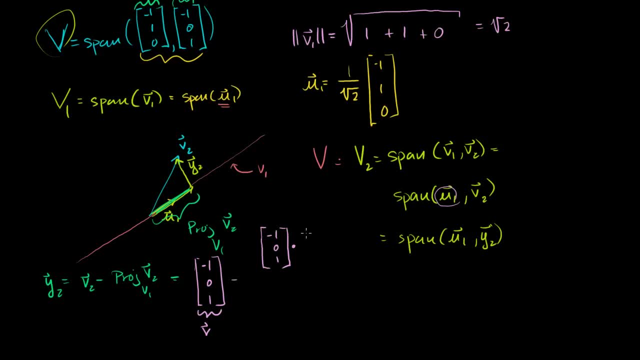 And we solved for u1 up here, So that's going to be that dotted with 1 over the square root of 2 times. let me do that in yellow actually, just so you can see that this is u1.. So dotting it with u1.. 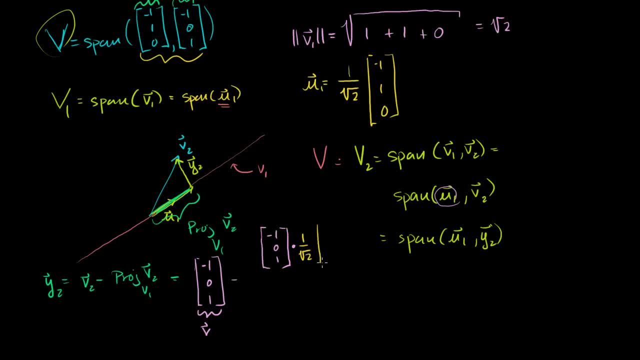 So dotting it with 1 over the square root of 2.. So 1 over the square root of 2 times minus 1, 1, 0.. I like leaving the 1 over the square root of 2 out of there. 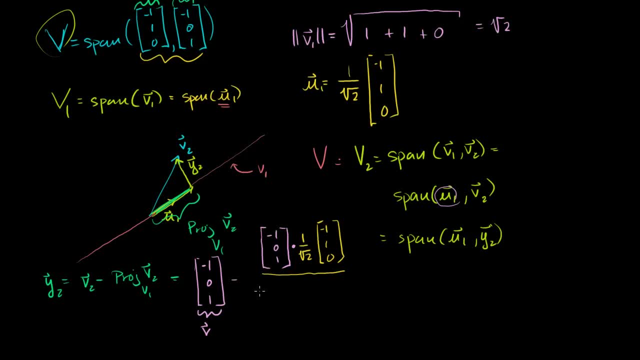 just to keep things simple, All of that divided by actually not divided by anything, because if we were doing a projection of a line, it would be divided by the dot product of the orthonormal basis with itself, but its length is 1.. 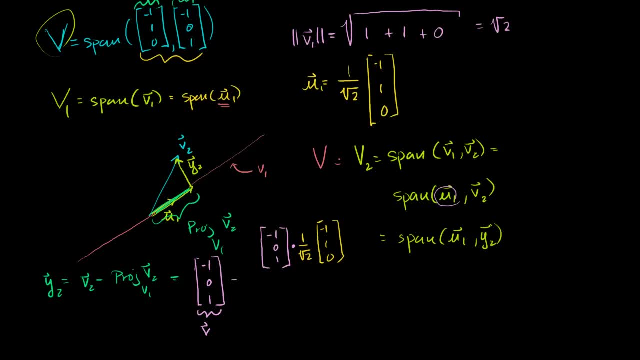 So we don't have that and we saw that before. So actually, let me write this a little bit. Let me write it a little bit. I'll just move it down. Let's see If I can move it. So it's just equal to that guy, right? 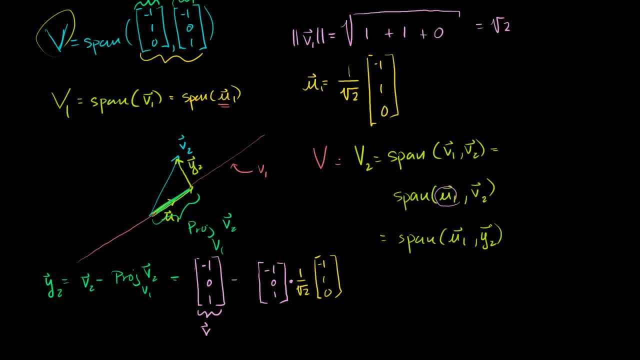 Let me make the numbers clear. This is v2 minus the projection of v2 onto the subspace 1. So that's just v2 dotted with my orthonormal basis for v1, my first vector in my orthonormal basis. 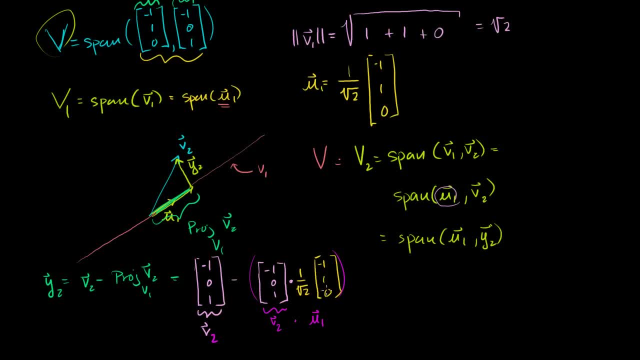 There's only one, so I'm only going to have one term here, And then all of that times my orthonormal basis, Orthonormal basis vector for v1.. So 1 over the square root of 2 times the vector minus 1, 1, 0.. 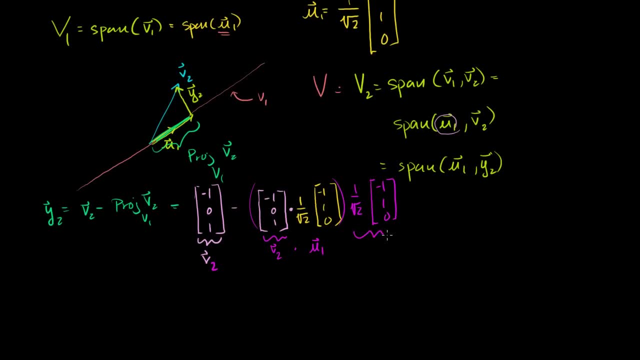 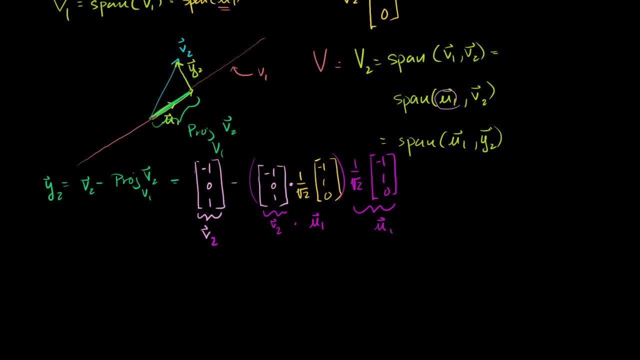 Now, this looks really fancy. This right here is our orthonormal basis for the subspace v1. But what does this simplify to? So this is going to be equal to remember this right here, this piece right there. that's the projection onto v1 of v2.. 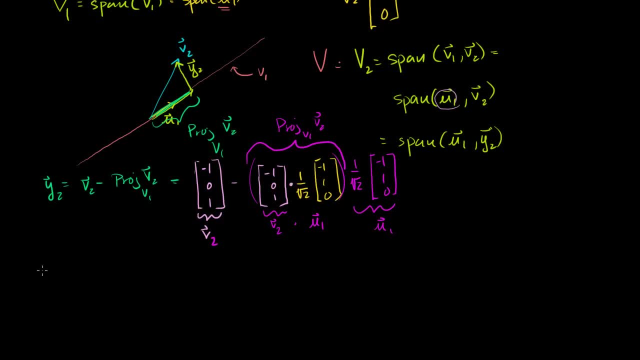 That's what that was right there. So this is going to be equal to the vector minus 1, 0, 1, minus. Now I could take the 1 over the square root of 2 on the outside. Actually, I could take both of these onto the outside. 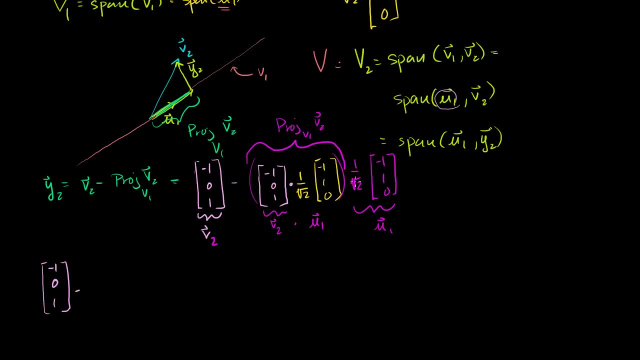 So 1 over the square root of 2 times 1 over the square root of 2 is just going to be 1 over 2.. So this is going to be minus 1 half times these guys dotted with each other. So what is? let me just write it this way: 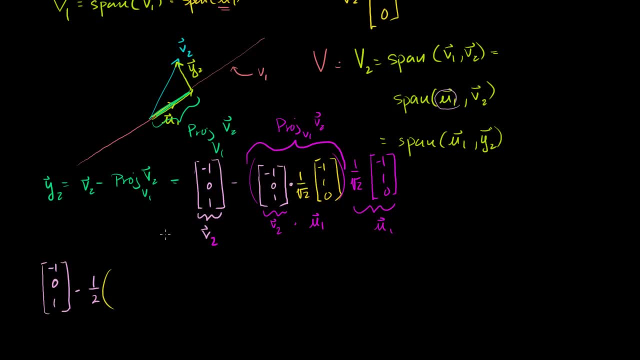 So what is these guys dotted with each other? It's going to be, It's just going to be a dot. It's just going to be a dot. It's just going to be a number. Minus 1 times minus 1 is 1, plus 0 times 1, so plus 0, plus. 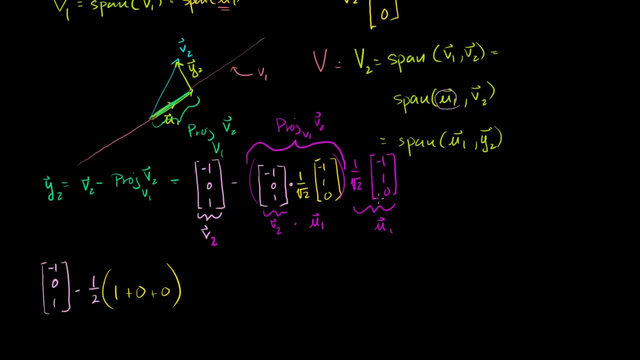 1 times 0,, so plus 0. All of that times. well, we already used this part of it, so we just have this part left over. Times minus 1,, 1, and 0.. This was the dot product and we took the two scaling. 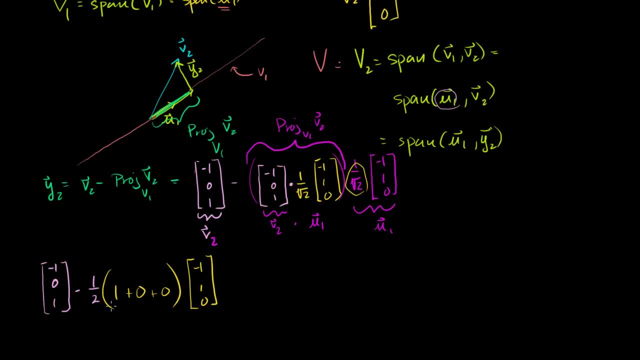 factors out. When you multiply them, you got a 1- half. So this is just going to be a 1, which simplifies things. So this is going to be equal to the vector minus 1, 0, 1, minus 1 half times this. 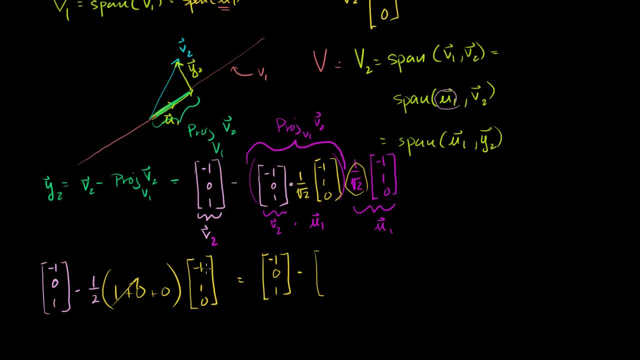 Or we could just write so: 1 half times minus 1 is minus 1 half. we have 1 half and then we have 0. And so this is going to be equal to minus 1, minus minus 1 half. that's plus 1 half, so that's going to be just minus. 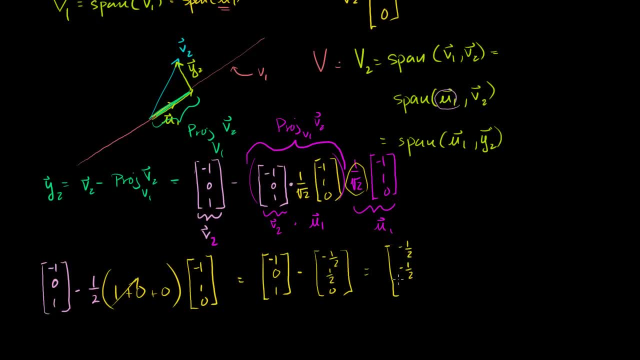 1 half. 0 minus 1 half is minus 1 half, and then 1 minus 0 is just 1.. So this right here is our vector y2.. And if you combine u1 right here and y2, we are spanning our. 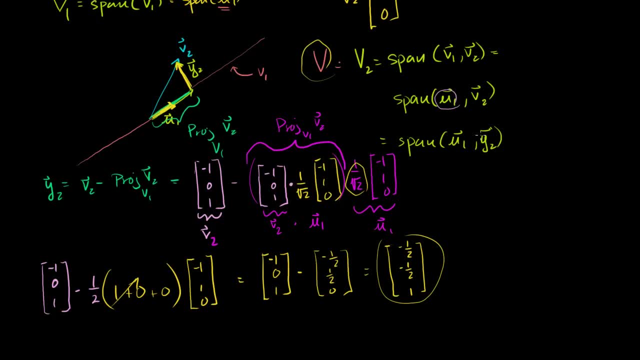 subspace V, But we don't have an orthonormal basis. These guys are orthogonal with respect to each other, but this guy does not have length 1 yet, So to make it equal to length 1, let's replace him. 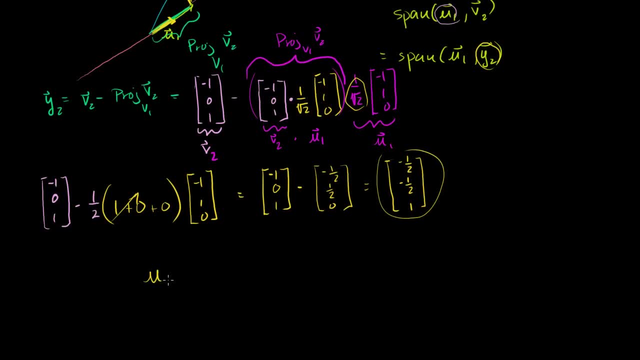 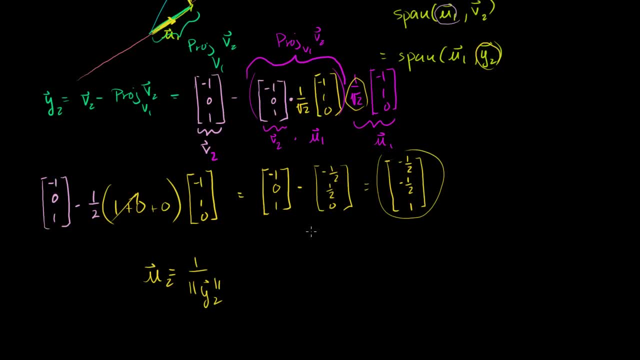 Let's define another vector, u2, that's equal to 1 over the length of y2.. 1 over the length of y2 times y2.. So what is the length of y2? The length of y2 is equal to the square root of minus 1 half. 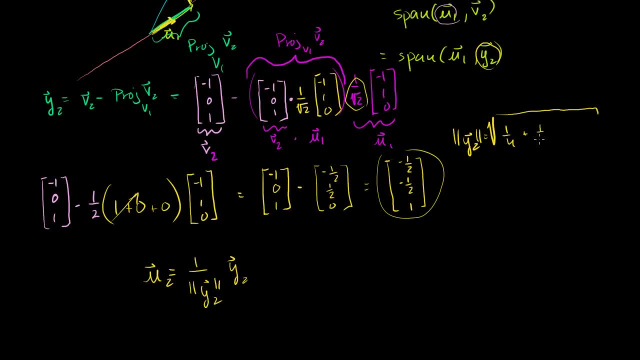 squared is 1 fourth plus 1 squared, So it's the square root of what is this? 1 and 1 half or 3 halves, So it's equal to the square root of 3 halves. This is 1 half plus 1 is 1 and 1 half, which is 3 halves. 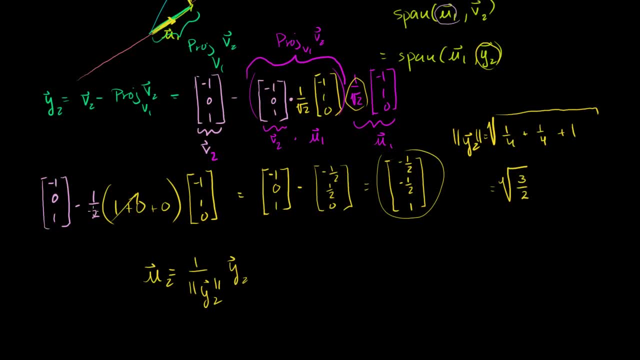 So it's equal to the square root of 3 halves. So if I define u2, u2 is equal to 1 over the square root of 3 halves, or that's the same thing as the square root of 2 thirds times y2, which is this guy right here minus 1 half. 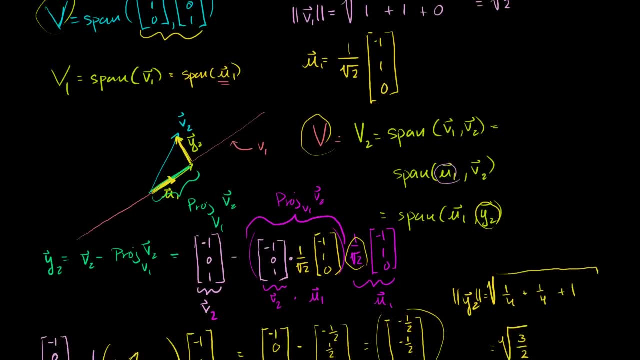 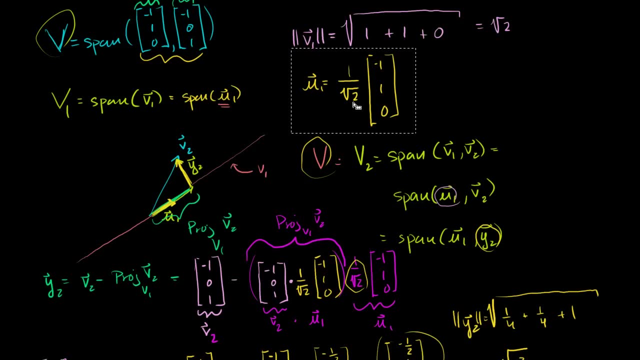 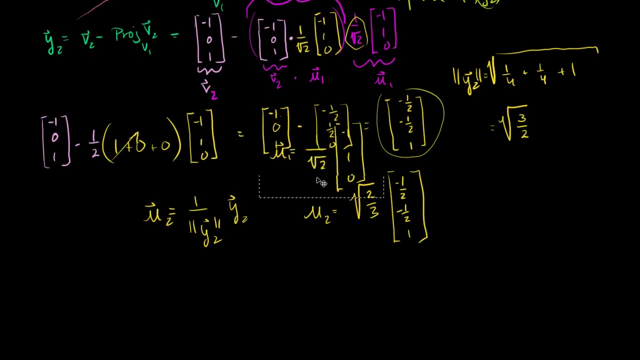 and 1. And I already had defined u1 up here. u1 was right up here. I can let me copy and paste. let me actually I can, just I think I can just move it down. So I found u1 right here. 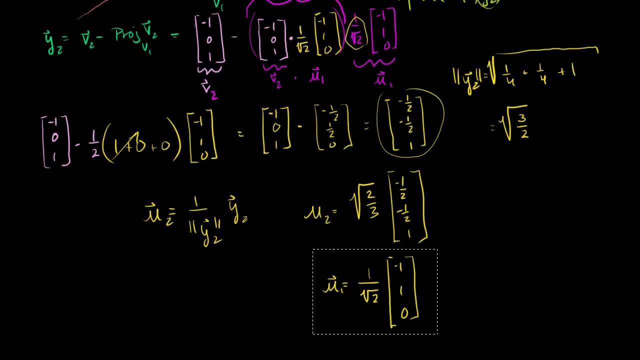 We now have two vectors that are orthogonal with respect to each other. So if I have the set of u1 and u2, these guys both have length 1. They're orthogonal. They're orthogonal with respect to each other And they span v. 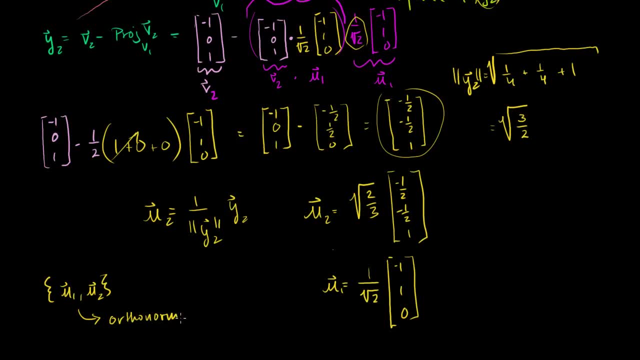 So this is an orthonormal basis for the plane that we started this video out with for v And we're done. We have done the Gram-Schmidt process. These are our new orthonormal basis vectors.